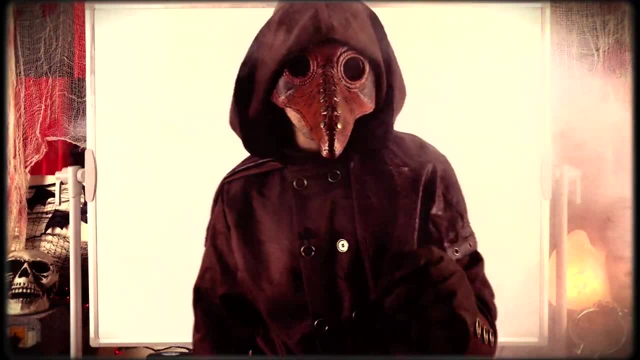 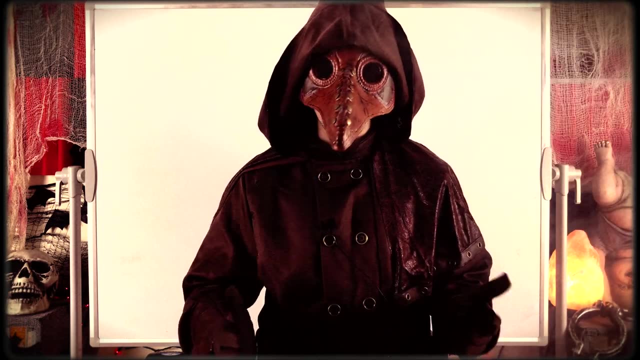 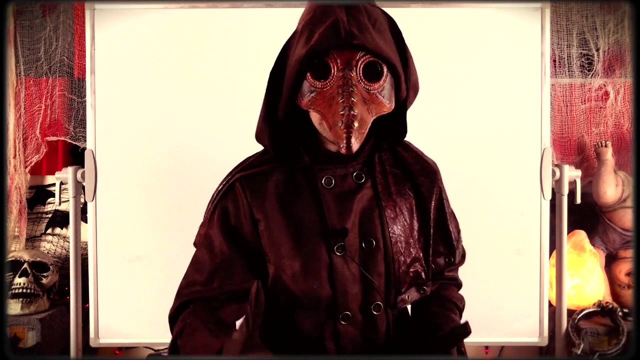 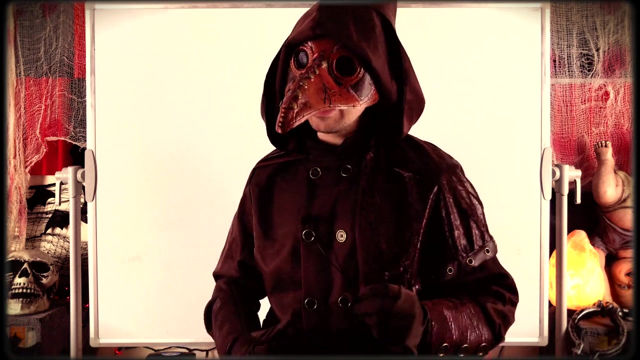 Good evening and welcome to another spooky Wrath of Math lesson. Tonight we'll be proving that set intersection distributes over set union. You're probably already familiar with the typical distributive property for multiplication and addition. We know that, for example, a times b plus c is equal to a times b plus a times c. The multiplication distributes over. 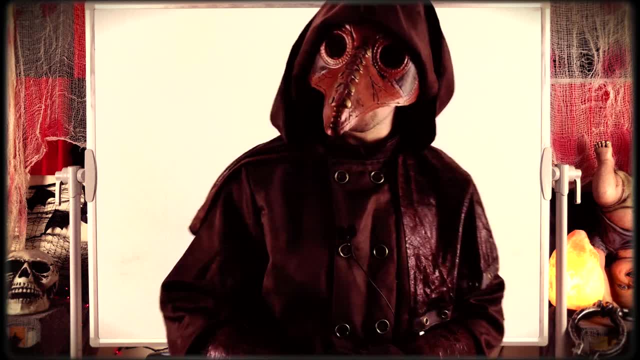 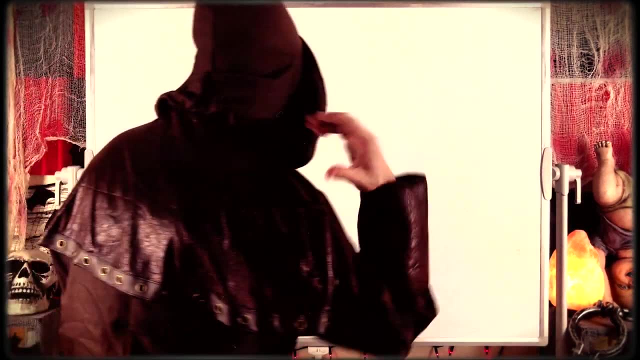 the addition Set intersection behaves in the same sort of way with set union, and that's what we'll be proving today. So let's just be super clear about what we are proving. Let me adjust my very spooky robe here, make sure that it's on correctly and let's write it out. 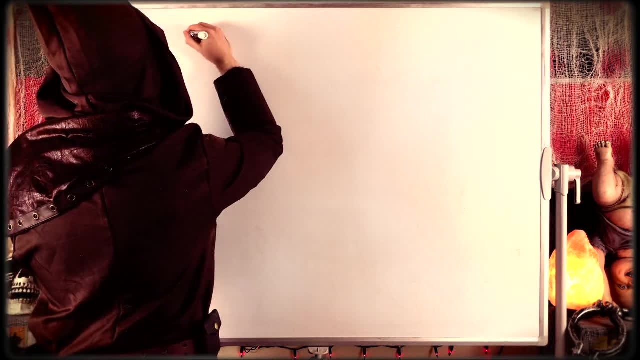 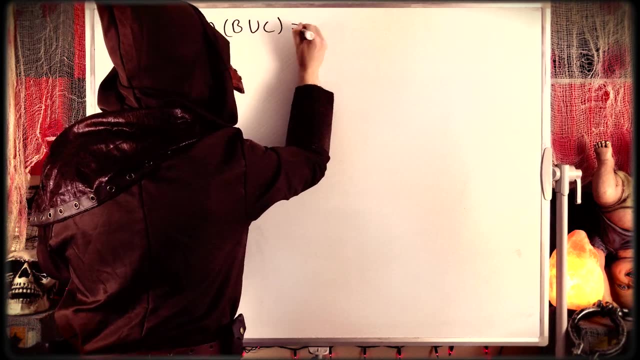 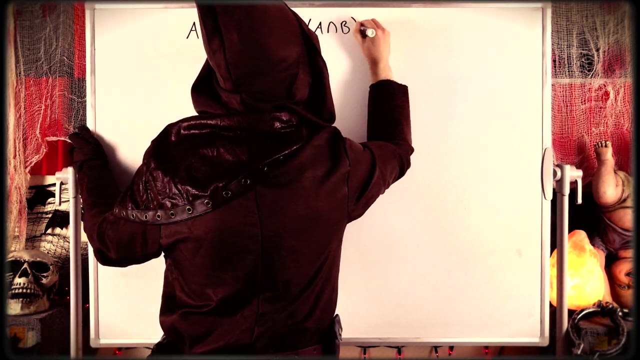 So what are we proving? We're proving that for three sets- a, b and c- a intersect b, union c. In this situation, intersection distributes over the set union so that this is equal to a intersect b unioned with a intersect c. 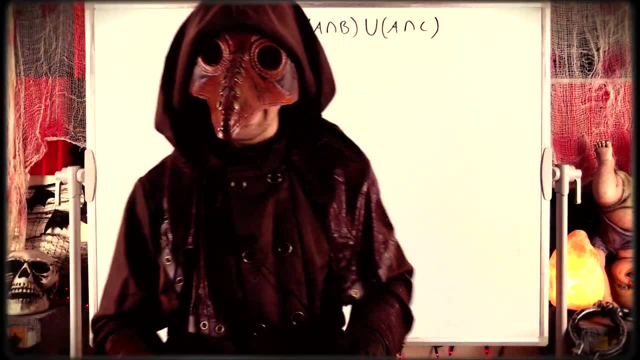 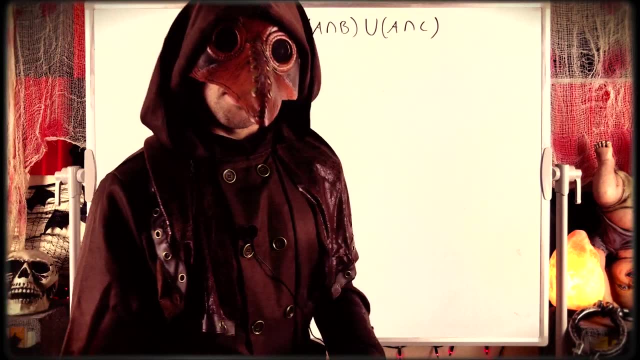 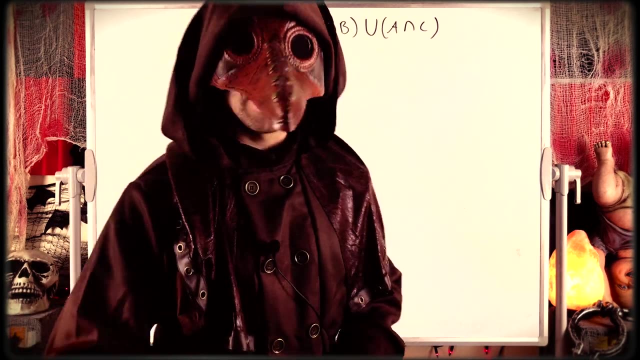 Just like that Works the same sort of way as multiplication and addition. As it turns out, union also distributes over set intersection this same way, which is pretty cool, and we'll prove that in another lesson. You can also give that a swing yourself after watching this one. 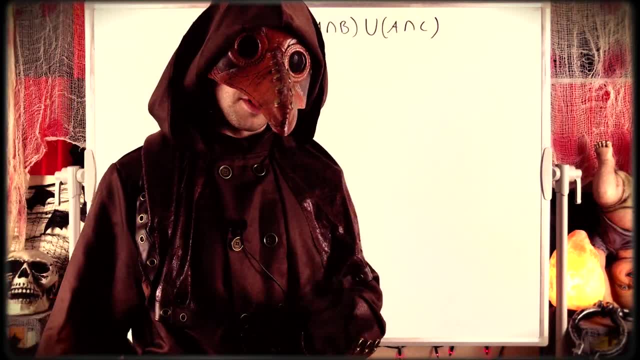 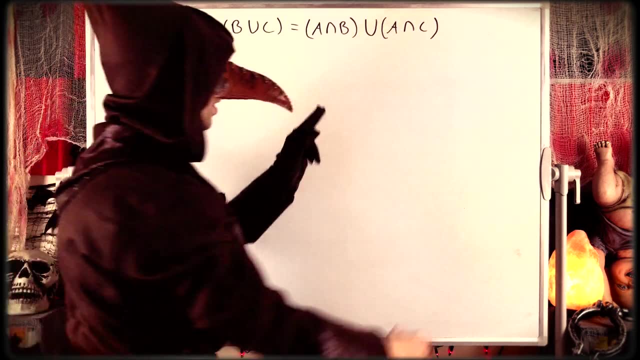 Now, it's a basic set equality proof. Remember to prove that two sets are equal. first, we'll need to show that this set is a subset of this set. then we'll need to show that this set is a subset of this set. It's all fairly straightforward. 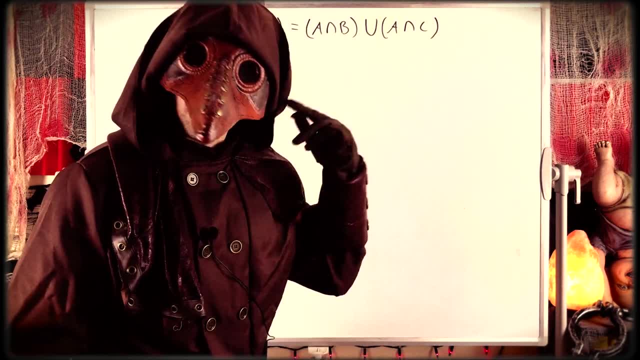 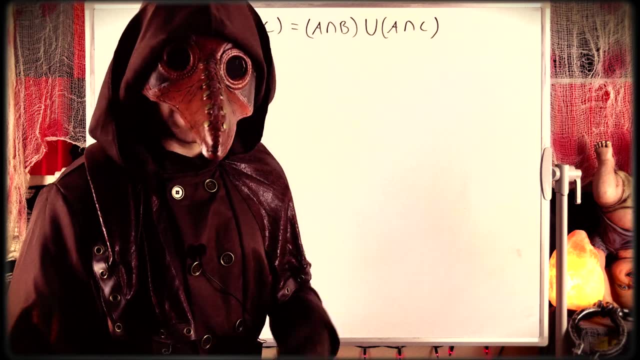 although it is a bit repetitious, which can make it difficult to understand by listening, because I'll be saying, you know, set and subset is an element of saying those things over and over again, which can sometimes make it a little tricky to follow. Before we get into that proof, 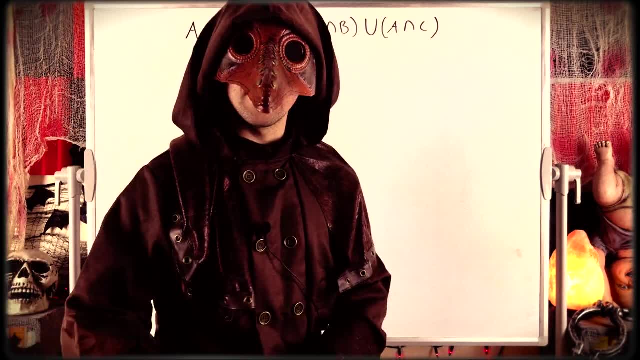 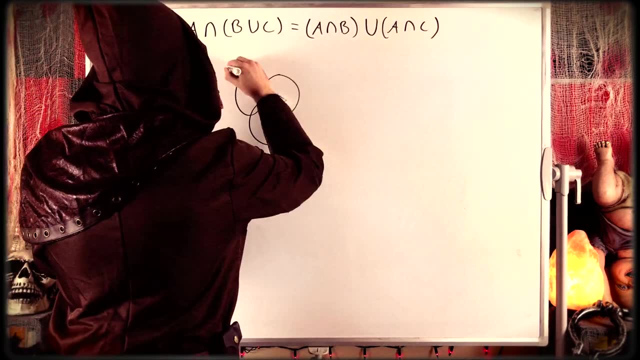 let's just see a Venn diagram, which will quickly convince us that this result is in fact true. So for the Venn diagram, we'll just have these three circles representing our sets a, b and c. What is a intersect b, union, c? 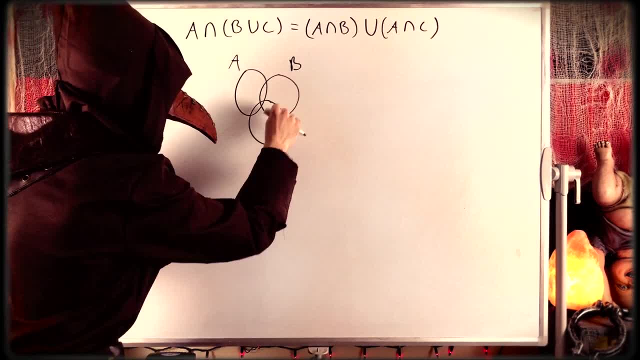 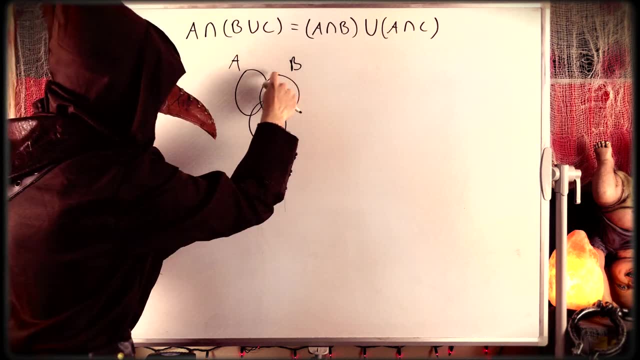 Well, b union c is b and c, all the stuff in those two sets. If we just take what is in common with b union c and a, that intersection, we just take what's in common with a, That's just going to be all of this stuff that I'm shading now. 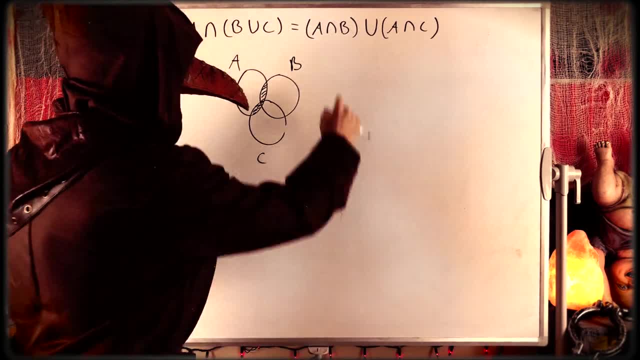 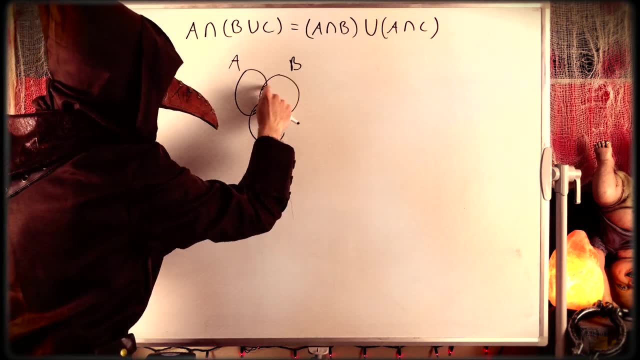 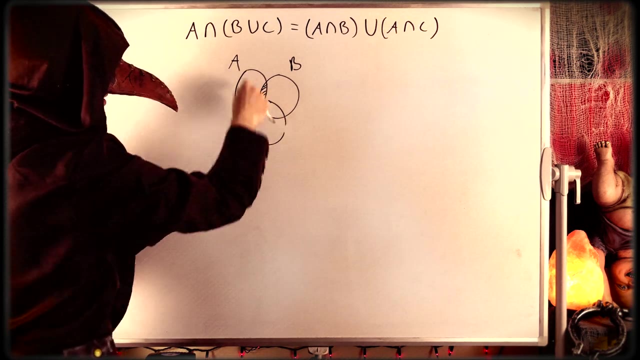 All right, so that's A intersect B- union C. What about this? What's A intersect B union A intersect C? Well, A intersect B is right there, A intersect C is right there And, oh look, if we union them, we get A intersect B union C, which we already shaded. 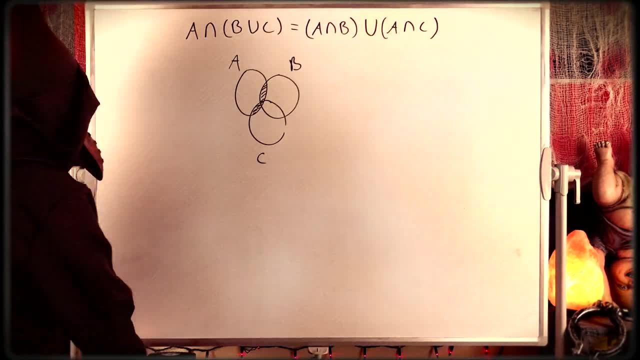 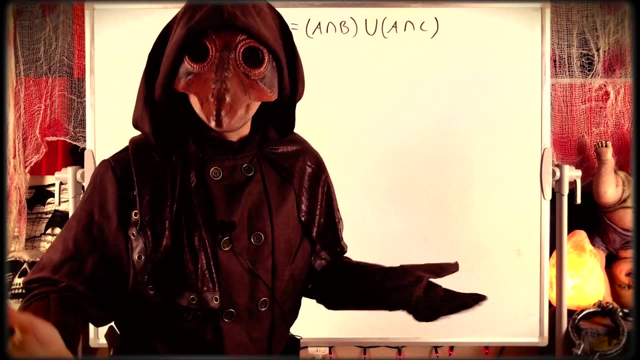 So we can quickly convince ourselves that, yes, this result is true. Now let's go ahead and get into the actual proof, which, again, is pretty straightforward but is, you know, a little monotonous. All right, first things. first, we want to show that this set is a subset of this set. 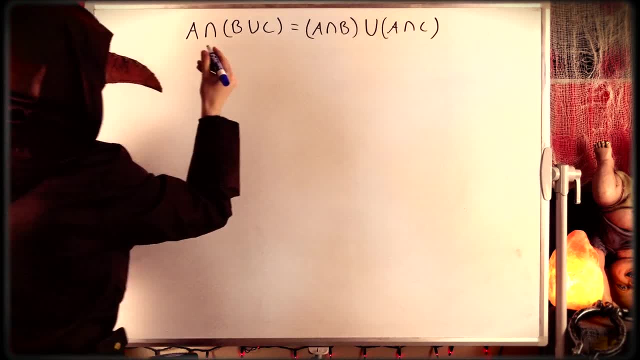 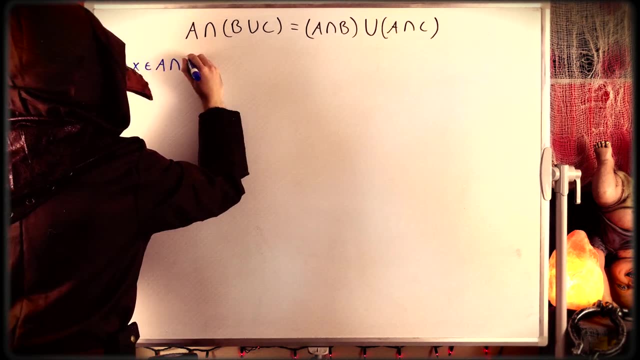 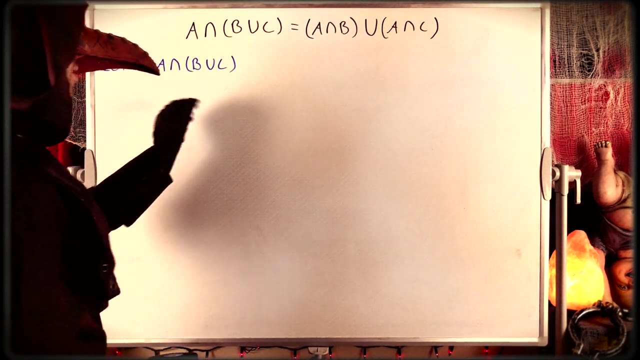 To do that, we begin with an arbitrary element from this set. So we'll say: let X be an element of our set. on the left: A, intersect B, union C. We just need to show that if we take any arbitrary, arbitrary element from this set, which is what we've just done- 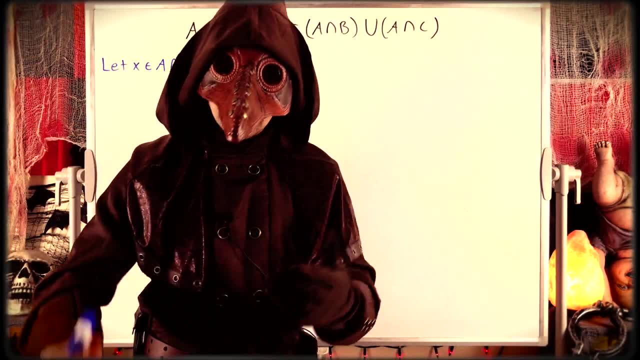 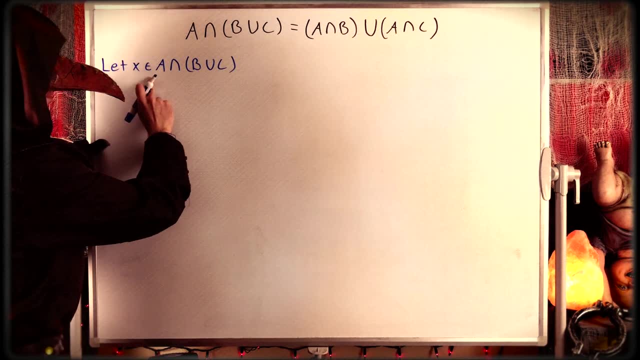 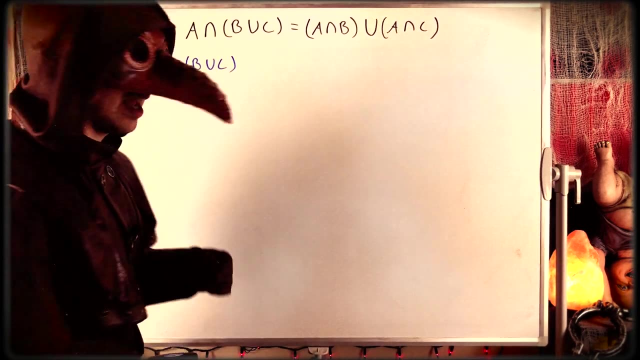 we need to show that it must also be an element of this set. That will prove our desired subset relation. So let's get into it. What do we know about X if it belongs to this set? Well, we know that certainly X has to be an element of A by definition of set intersection. 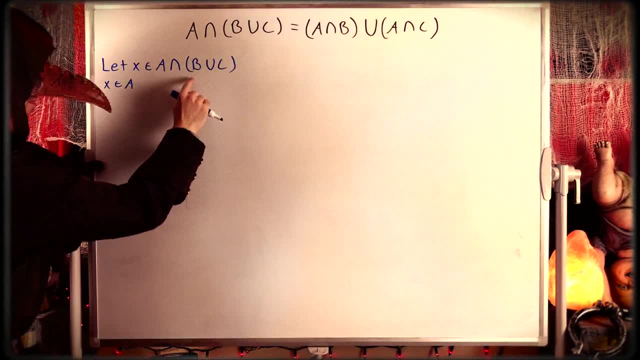 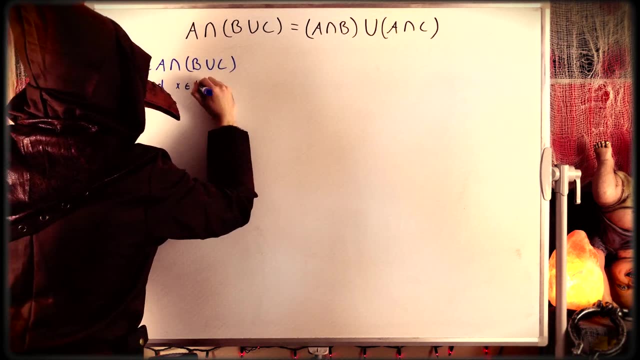 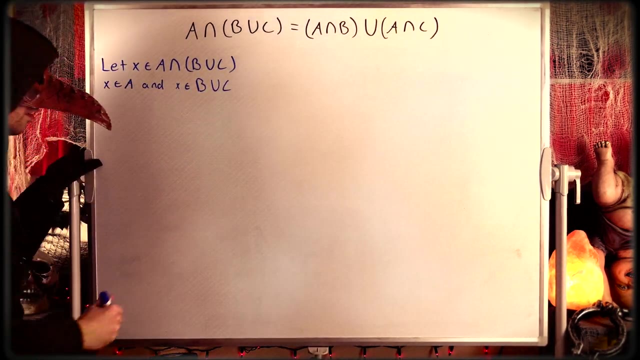 X has to be an element of A and X has to be an element of B union C. So we could write that here X is an element of A and X is an element of B union C. Okay, now what does this mean for X to be an element of B union C? 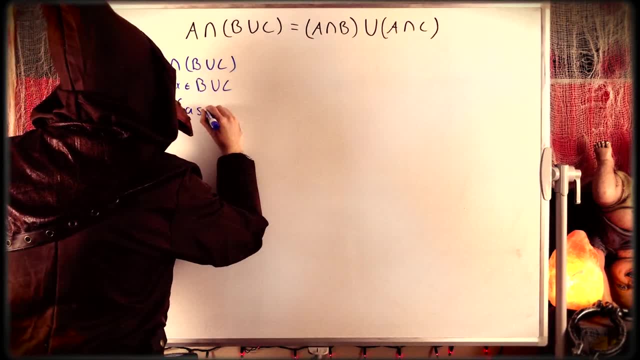 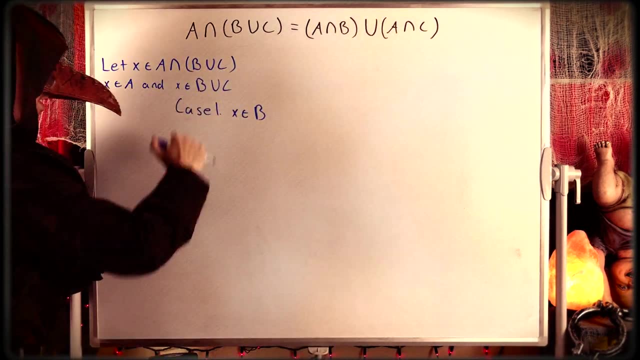 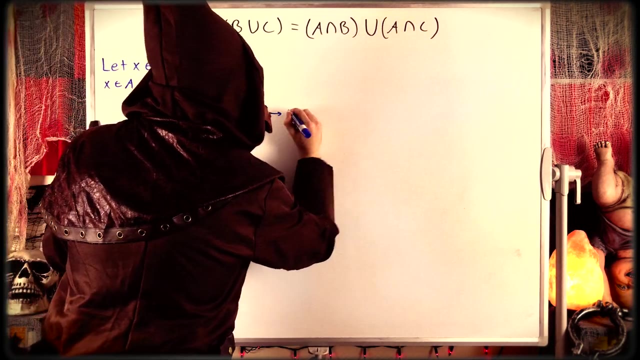 Well, there are basically two cases. Case one would be that X is an element of B. If X is an element of the set B, well we know that X is an element of A. So if X was also an element of B, that would mean that X. 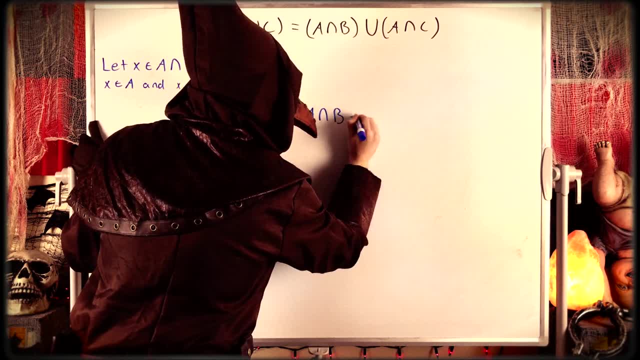 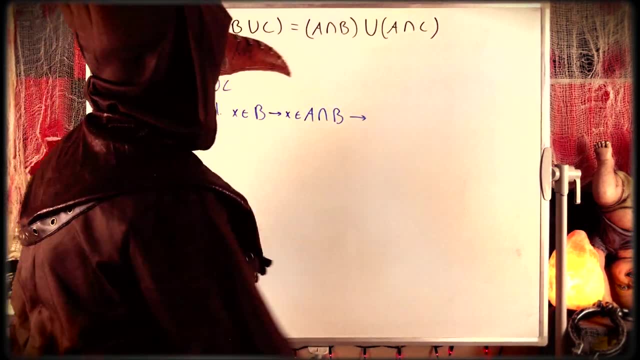 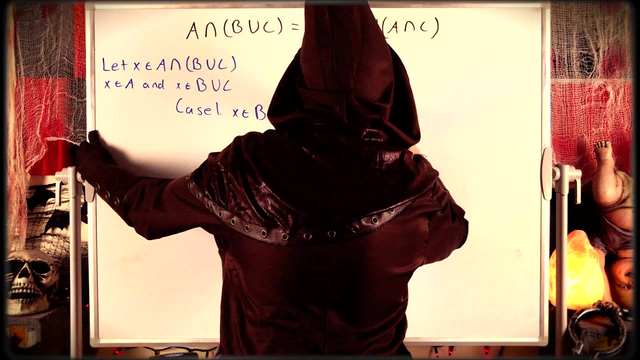 is an element of A intersect B. Thus, by definition of set union, if X is an element of A intersect B, then X is an element of A intersect B union A intersect C, And so we'll write that here. This would imply that X, by definition of set union, 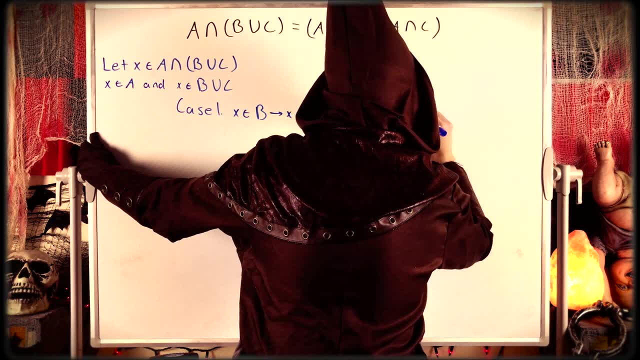 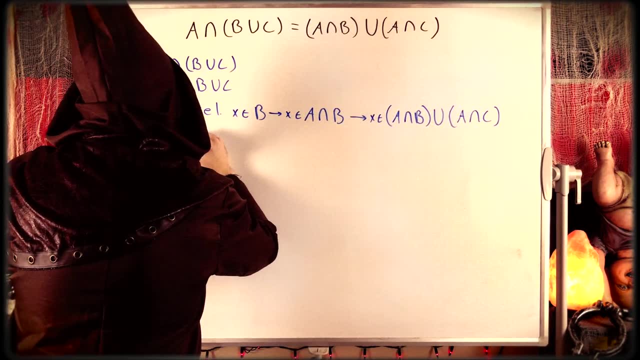 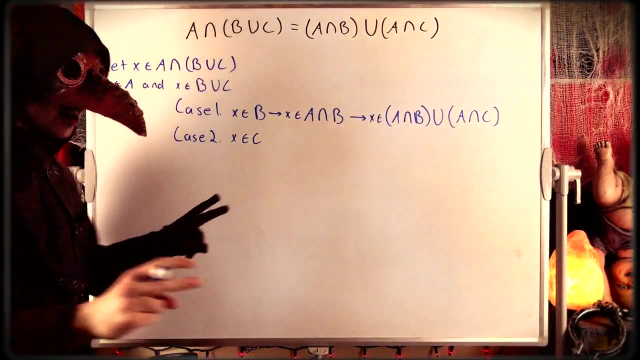 has to be an element of A intersect B, union A intersect C. All right. Case two Goes basically the exact same way. Case two would be that X is an element of C. Now there is a sort of third case where X is an element of both B and C. 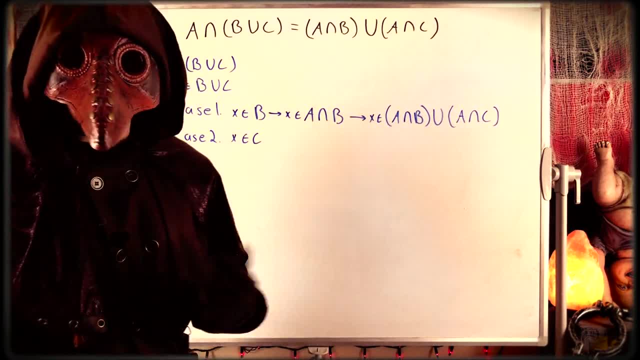 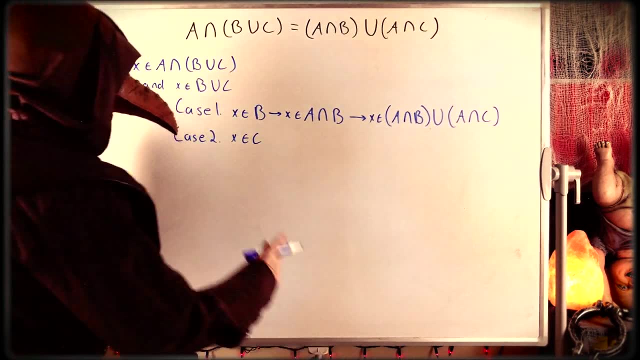 But note that case is covered by both of these cases. If X is an element of B and C, then case one applies and so does case two. So we're still covered. There's only two cases we have to think about. If X is an element of C, what do we know? 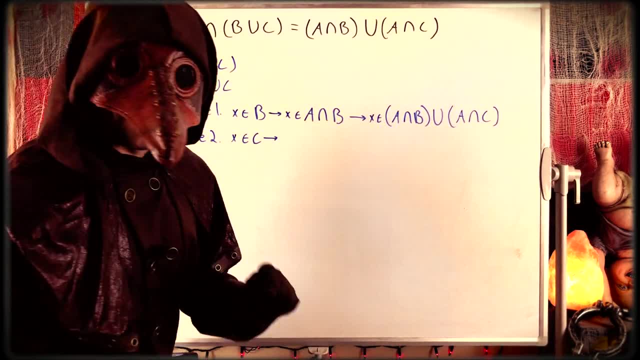 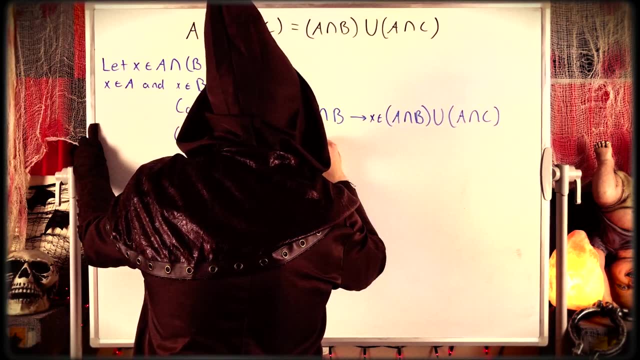 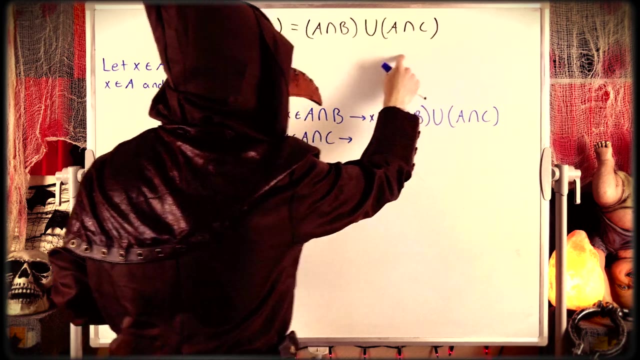 Same sort of thing. We're guaranteed that X is an element of A. So if X is an element of C, then X is an element, by definition of set, intersection of A, intersect C, Then by definition of set union. if X is an element of this set, X is an element of that set. 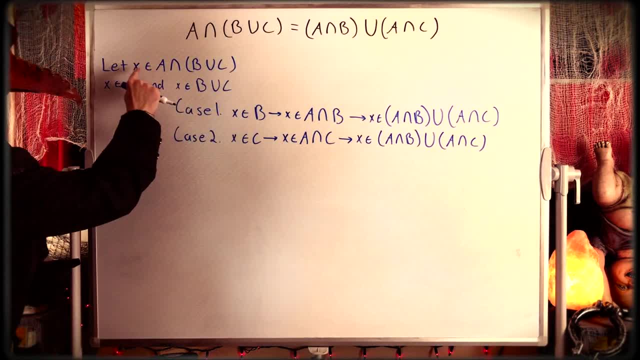 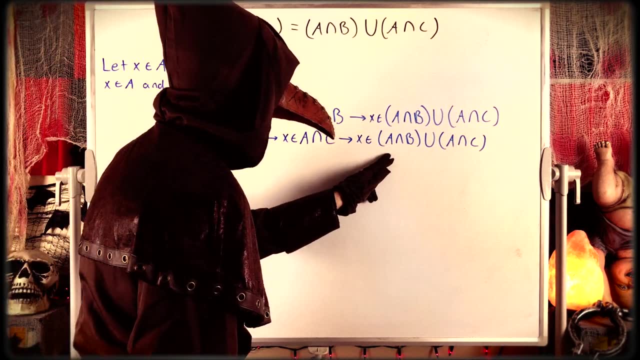 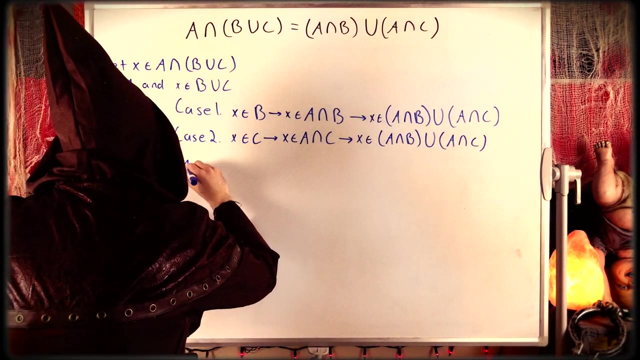 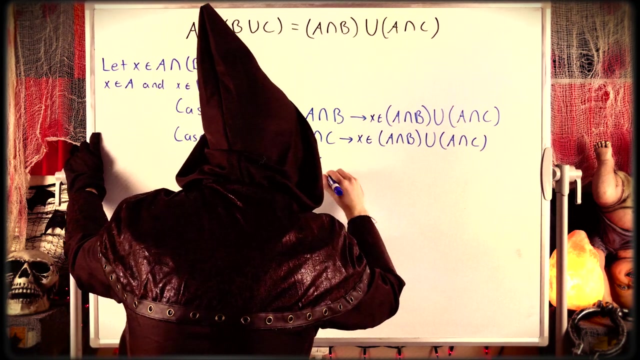 And so we see we are guaranteed. if we take an arbitrary element from A intersect B union C, it must be the case that element is also an element Of A intersect B union A intersect C. Thus, by definition of subset we have our desired subset relation: that A intersect B union C must be a subset of A intersect B union A intersect C. 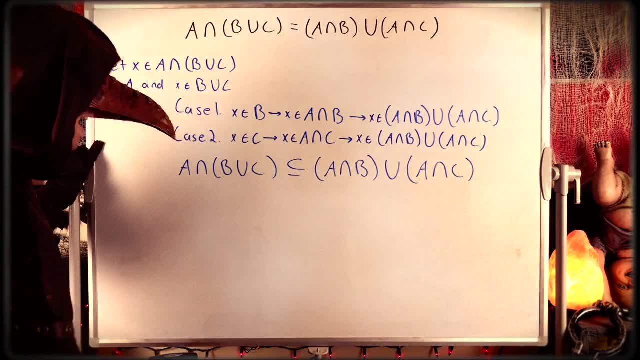 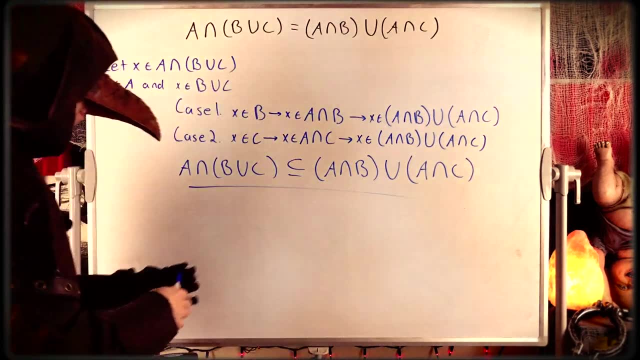 Because we just showed. we just showed that any element of this set also has to be an element of that set. So we get our desired subset relation. Now the second part of the proof. We just have to show that this set is also a subset of this set, and then we'll be done. 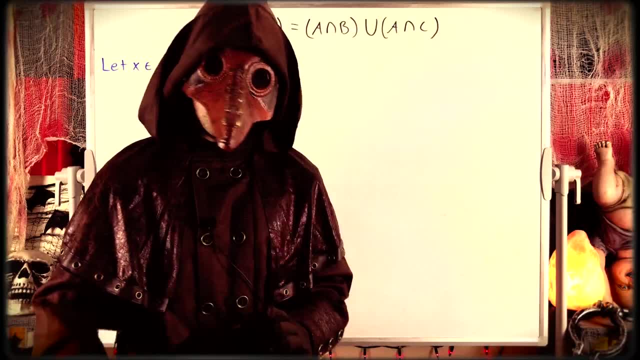 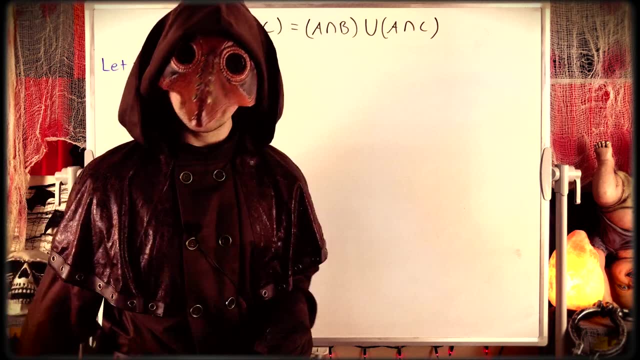 We will have our desired set equality. All right, So I erased most of what was on the board, So we got some more room to work with. You can, of course, rewind the video if you want to take another close look at what we had previously written. 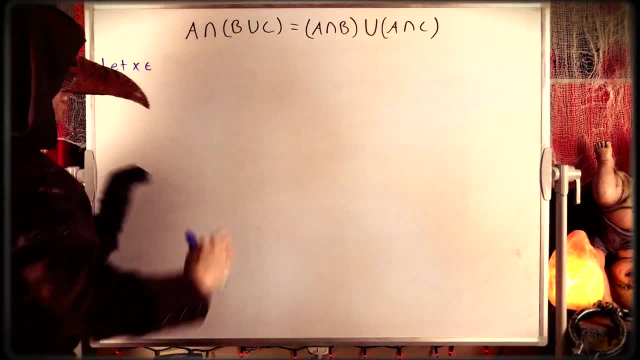 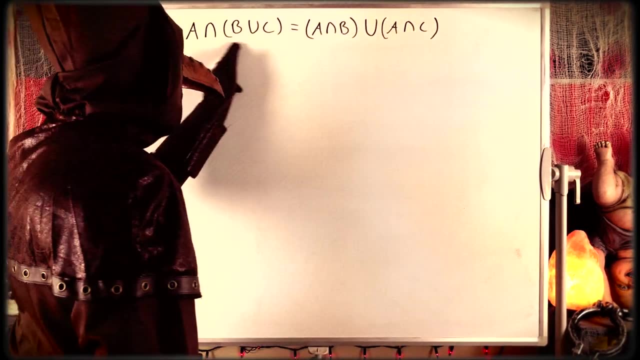 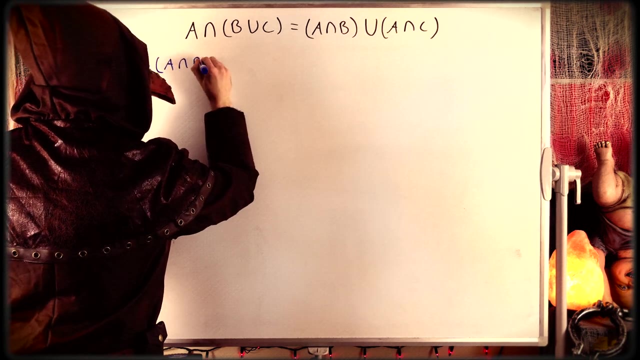 Again. now we want to show that this is a subset of this. So we begin by taking an arbitrary element from this set and we just have to show that element must also belong to this set. So we'll say: let X be an element of A intersect B, union A intersect C. 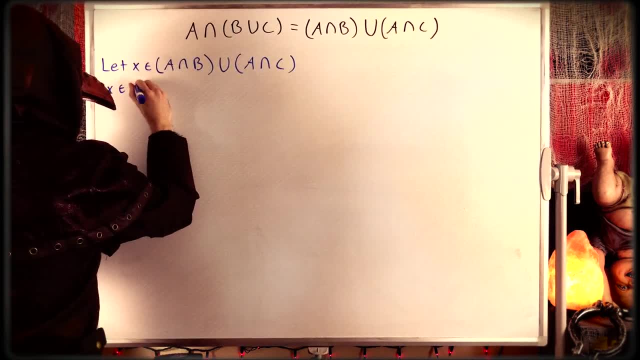 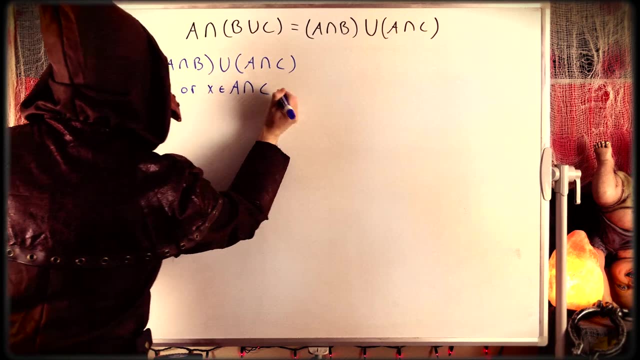 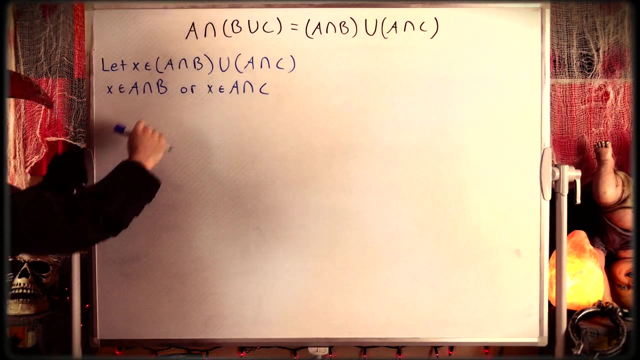 Now this means, by definition of set union, that X is an element of A intersect B or X is an element of A intersect C. This basically gives us a two case situation. Again, we could have case one: X is in A intersect B. 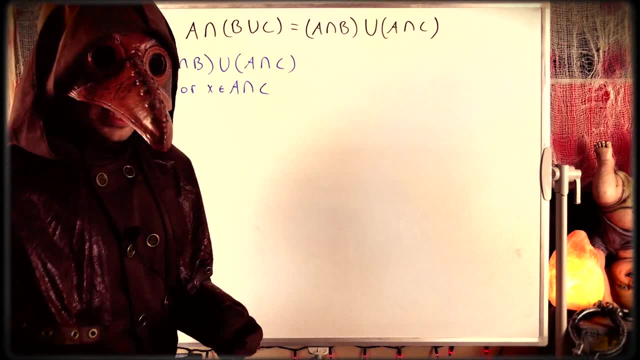 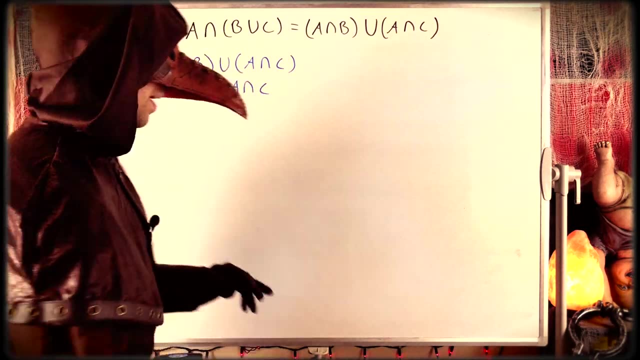 Or case two: X is in A intersect C. There's a sort of case three again, where X is in both of these sets. But if X is in both sets, then it's covered by each of the individual cases that we're looking at. 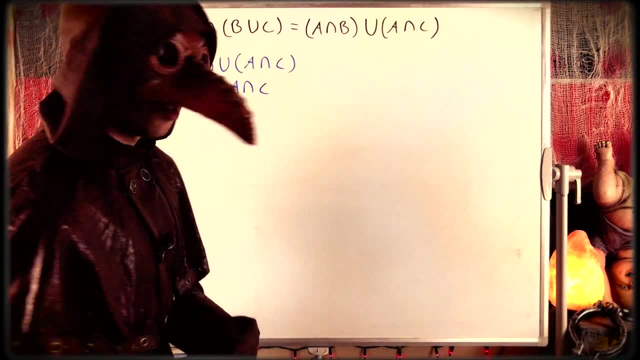 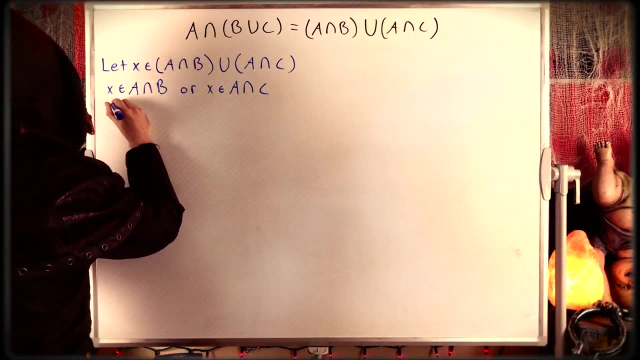 So let's say that X is an element of A intersect B. What does that mean? Well, that would mean that X is an element of A. So we could write that underneath here: X is an element of A, and it means, of course, X is an element of B. 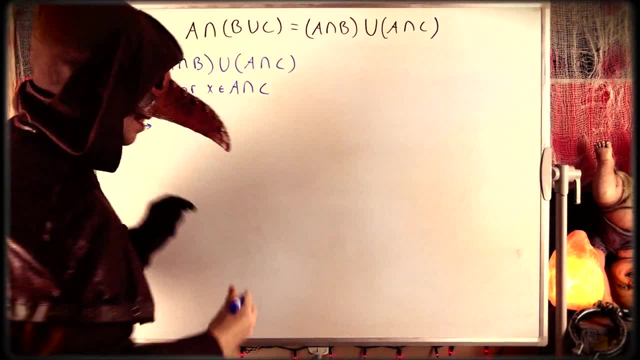 But if X is an element of A, then it means that X is an element of B. But if X is an element of A, then it means, of course, X is an element of B. But if X is an element of B, then by definition of set union, that would mean that X is an element of B. union C: 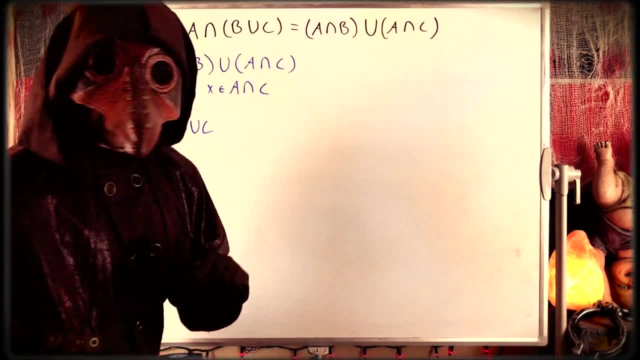 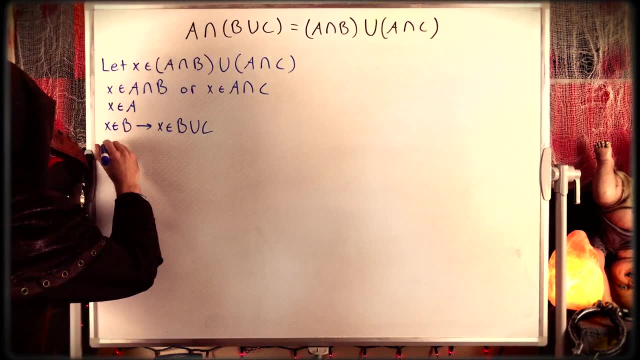 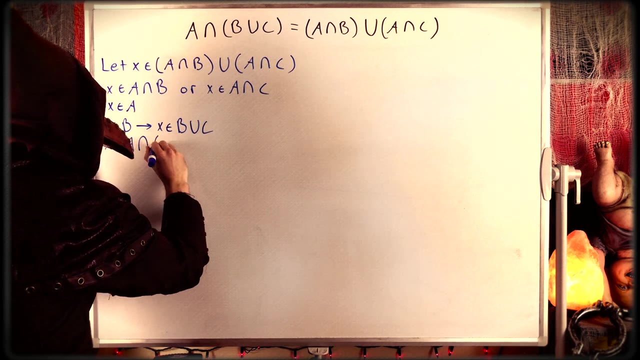 Oh look, so that means if X is in A intersect B, that means that X is in A and X is in B union C. Thus, by definition of set intersection, we would have our desired result that X is an element of A intersect B union C. 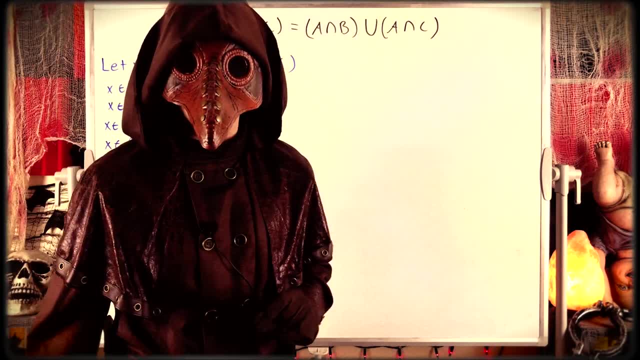 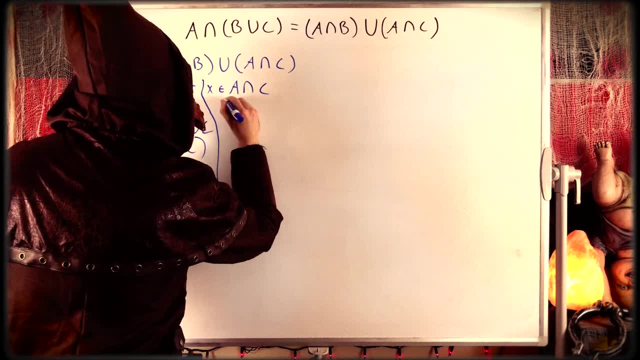 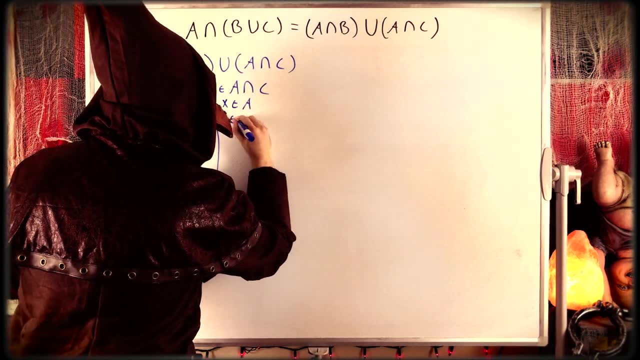 So case two: let's say that X is an element of A intersect C, element of A intersect C. That means, by definition of set intersection that A, excuse me, that X is an element of A. it also means that X is an element of C. But if X is an element of C, then by definition.